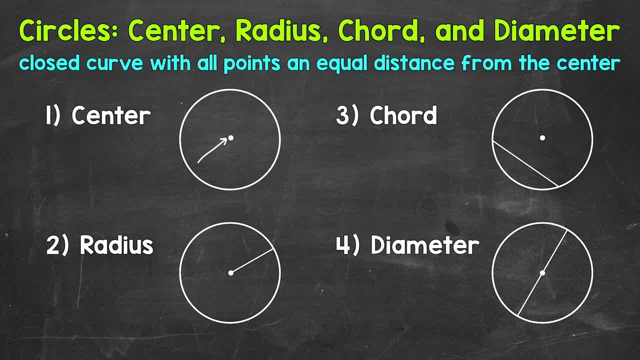 on the circle is the exact same distance from the center. Now you may see a letter next to the center of a circle, For example. let's put an A here next to the center, And that letter is going to be how we name a circle. We name a circle by. 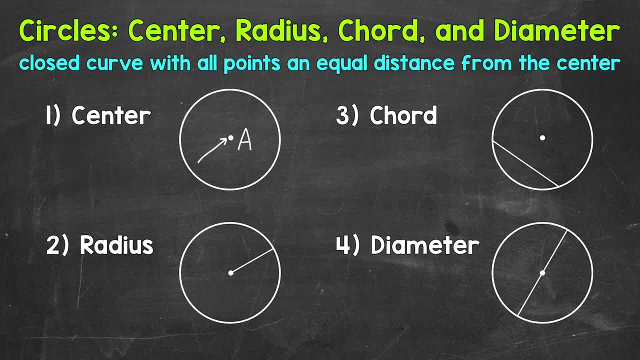 its center. So this would be circle A. I do have another video that goes into further detail on how to name a circle and parts of a circle. That link is down in the description. Let's move on to radius, which is the distance from the center of the circle to any point. 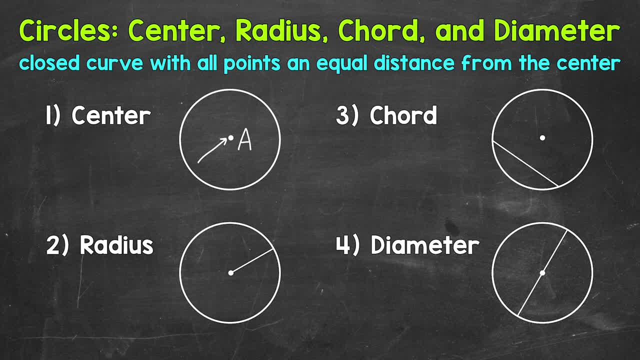 on the circle itself, So the length of a line segment that connects the center to any point on the circle. For example, we go from the center right here to this point on the circle. Now we can actually have more than one radius. For example, we can go from the center. 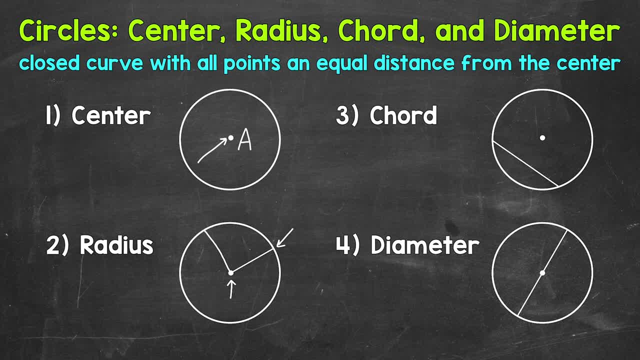 to this point, this point on the circle right there, The plural form of radius is radii. Let me write that out. So the plural form of radius is radii. Now, keep in mind, no matter how many radii you have, or 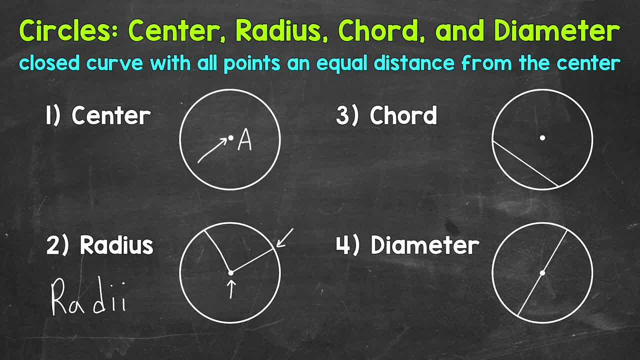 what direction they are going, meaning from the center to whatever point on the circle they are going, they will all have the same measure. They are all congruent Because, remember, all points on a circle are the exact same distance from the center. So, for example, if this radius right here, 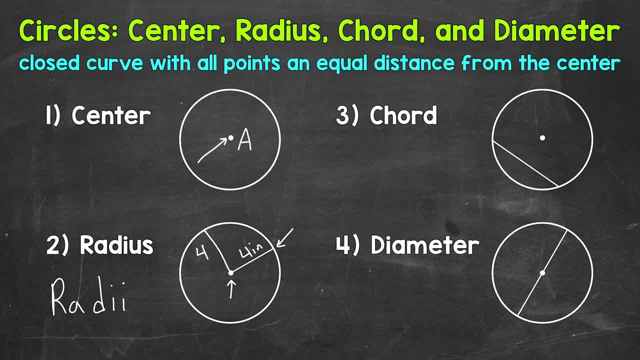 is four inches- this one over here will be as well, and any other radii within that circle. So again, radius. we are going from the center to any point on the circle. Next we have chords, And a chord is a line segment that connects two points on the circle. 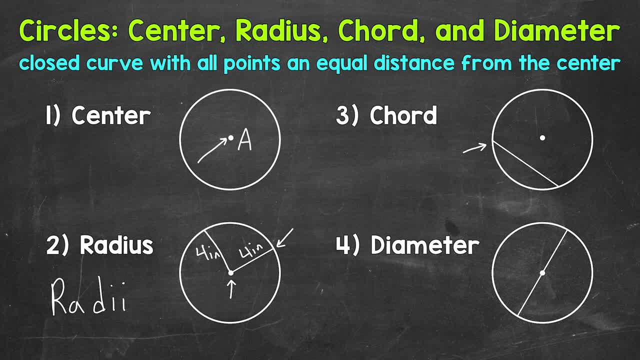 So one point right here and a line segment to another point on the circle right here. So we have a line segment that connects two points on the circle. There's no particular direction or positioning of the points that are connected, just the fact that two points. 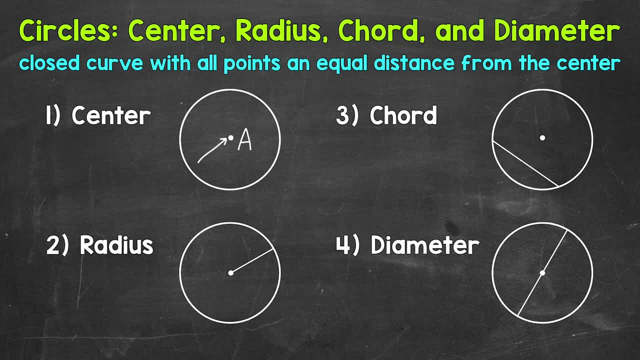 its center. So this would be circle A. I do have another video that goes into further detail on how to name a circle and parts of a circle. That link is down in the description. Let's move on to radius, which is the distance from the center of the circle to any point on the 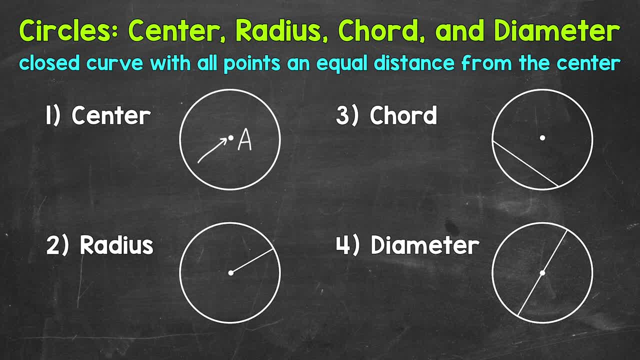 circle itself, So the length of a line segment that connects the center to any point on the circle. For example, we go from the center right here to this point on the circle. Now we can actually have more than one radius. For example, we can go from the center. 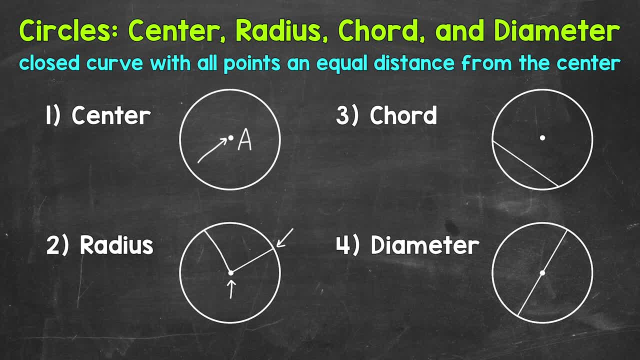 to this point, this point on the circle right there, The plural form of radius is radii. Let me write that out. So the plural form of radius is radii. Now, keep in mind, no matter how many radii you have, or 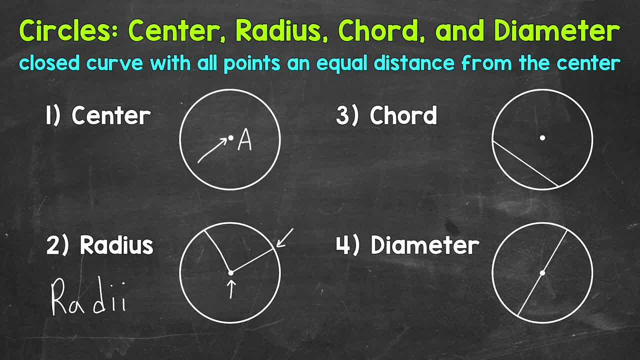 what direction they are going, meaning from the center to whatever point on the circle they are going, they will all have the same measure. They are all congruent Because, remember, all points on a circle are the exact same distance from the center. So, for example, if this radius right here, 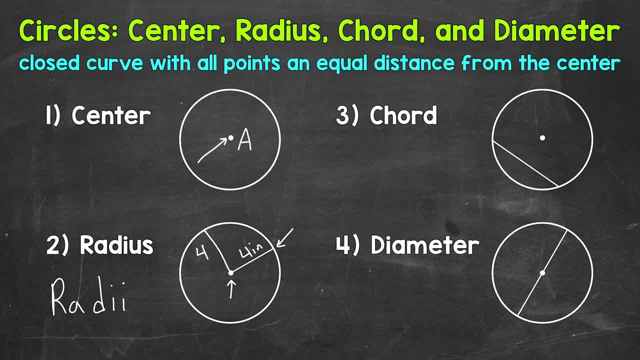 is four inches- this one over here will be as well, and any other radii within that circle. So again, radius. we are going from the center to any point on the circle. Next we have chords, And a chord is a line segment that connects two points on the circle. 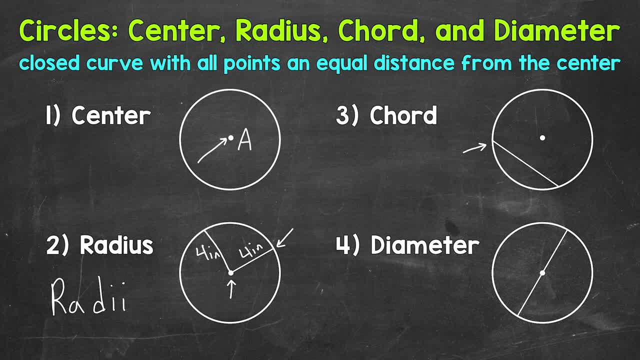 So one point right here and a line segment to another point on the circle right here. So we have a line segment that connects two points on the circle. There's no particular direction or positioning of the points that are connected, just the fact that two points. 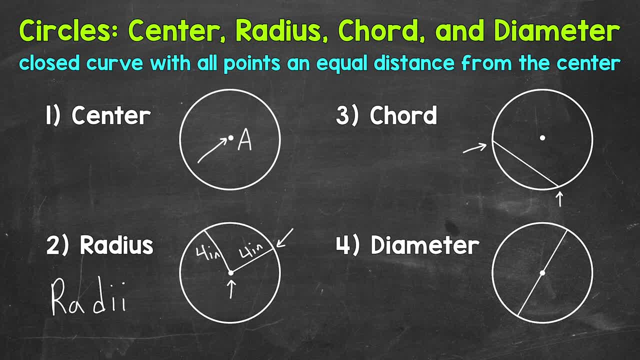 on the circle are connected. So we have a line segment that connects two points on the circle. There's no particular direction or positioning of the points that are connected, just the fact that two points on the circle are connected. And that's going to be a chord. 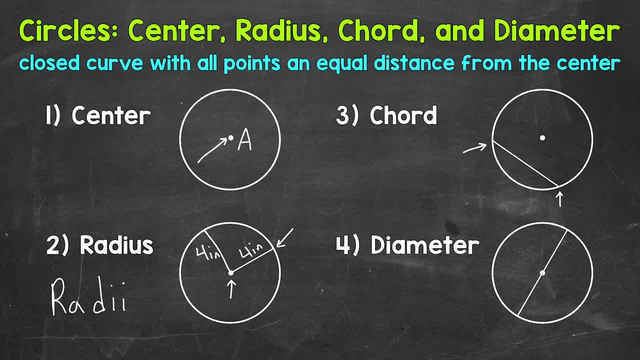 Let's draw out another example of a chord before moving on, So we could go from here, the top of the circle, down to another point on the circle, And that will give us another example of a chord. Lastly, let's move on to diameter. Now, diameter is a very specific type of chord. 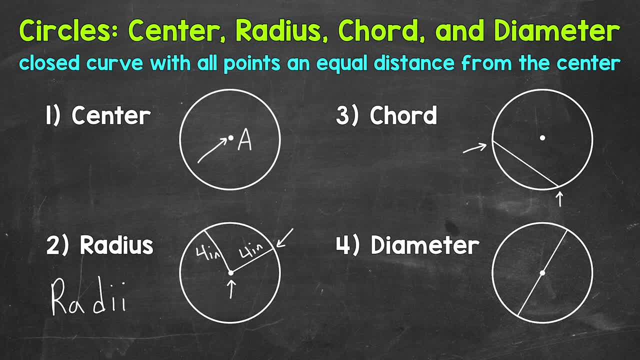 on the circle are connected. So we have a line segment that connects. two points on the circle are connected And that's going to be a chord. Let's draw out another example of a chord before moving on. So we could go from here, the top of the circle, down to 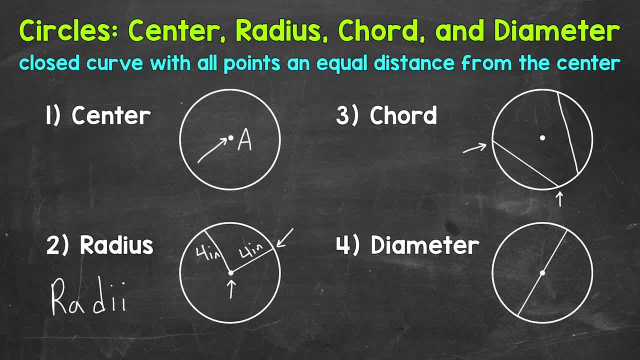 another point on the circle, And that will give us another example of a chord. Lastly, let's move on to diameter. Now, diameter is a very specific type of chord. It's a line segment that connects two points on the circle, but it has to. 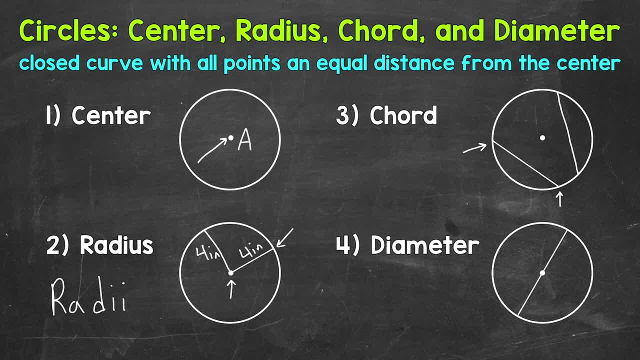 go through the center of the circle. So, for example, we have a line segment that connects this point and this point on the circle and goes through the center. A diameter is actually the longest chord possible because it goes all the way across the circle. A diameter cuts or divides a circle in half, so two equal. 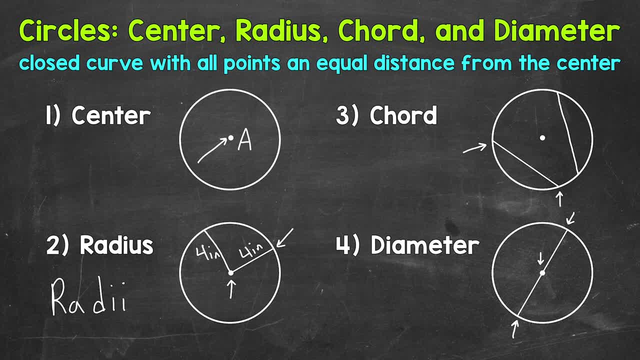 parts. Each part or half is called a semicircle. Another important thing to understand about diameters is that they are twice the length of the radius, or vice versa. The radius is half the diameter, For example, since all of the 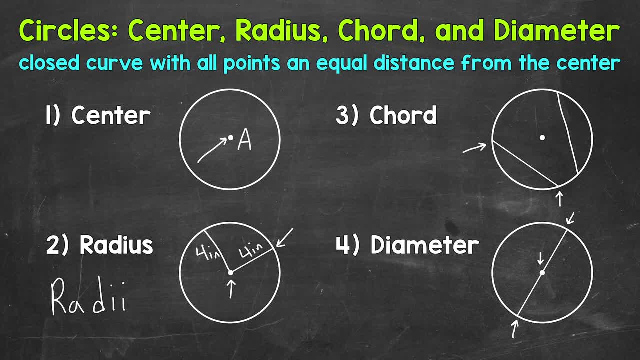 circles in this video are the same size. if the radius is 4 inches, take a look at number 2,. that means that the diameter will measure 8 inches Because, again, the diameter is twice the radius. So this diameter here is going to be 8 inches. 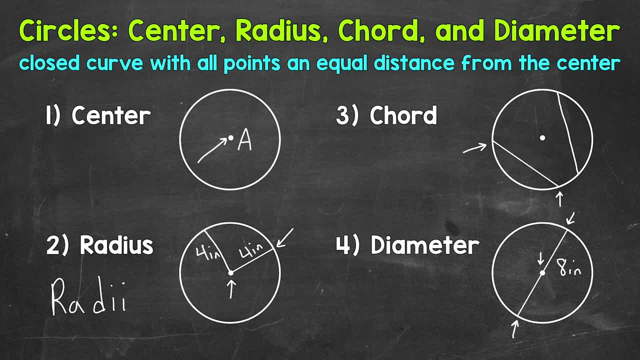 And one last thing I do want to mention about diameters is that it does not matter what direction a diameter is going, as long as it connects two points on the circle and goes through the center. So there you have it. There is an overview of four very important parts of a circle. 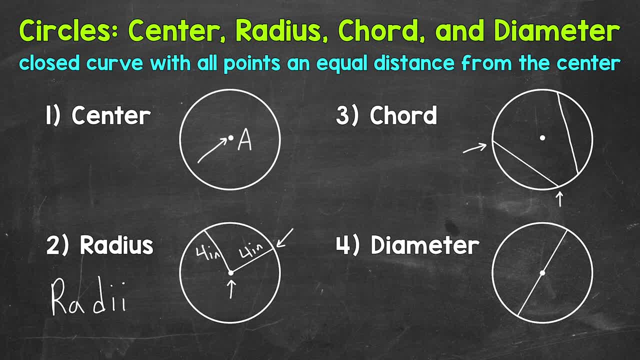 It's a line segment that connects two points on the circle. But it's a line segment that connects two points on the circle- But it's a line segment that connects two points on the circle- has to go through the center of the circle. So, for example, we have a line 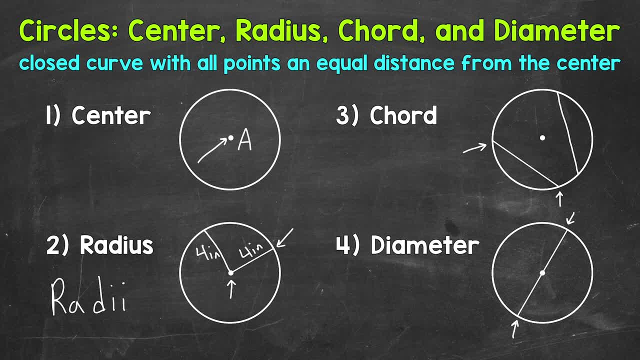 segment that connects this point and this point on the circle and goes through the center. A diameter is actually the longest chord possible because it goes all the way across the circle. A diameter cuts or divides a circle in half, so two equal parts. Each part or half is called a semicircle. 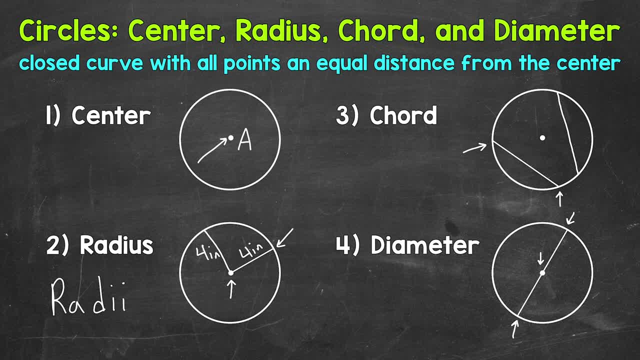 Another important thing to understand about diameters is that they are twice the length of the radius, or vice versa. The radius is half the diameter. For example, since all of the circles in this video are the same size, if the radius is four inches, take a look at number two. that means that the diameter will 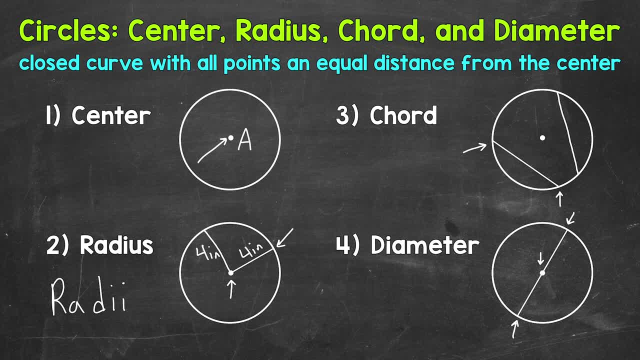 measure eight inches because, again, the diameter is twice the radius. So this diameter here is going to be eight inches. And one last thing I do want to mention about diameters is that it does not matter what direction a diameter is going, as long as it connects. 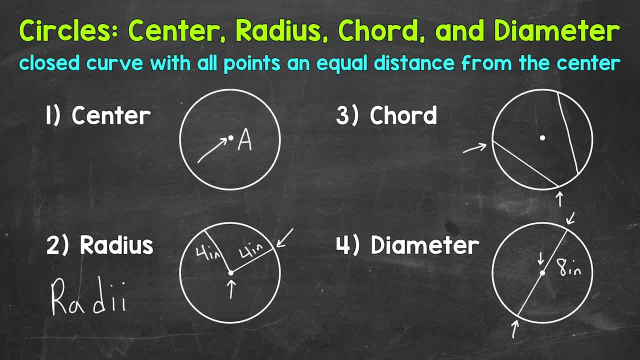 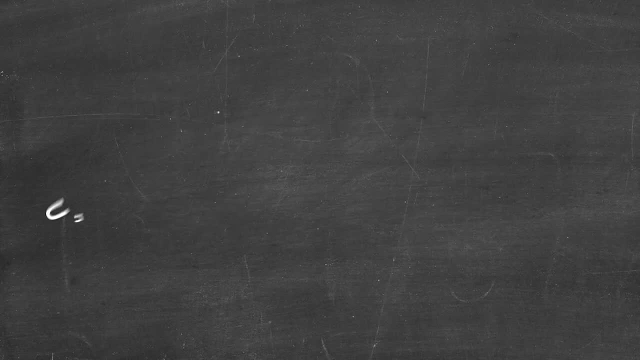 two points on the circle and goes through the center. So there you have it. There is an overview of four very important parts of a circle: Center: radius, chord and diameter. I hope that helped. Thanks so much for watching In.